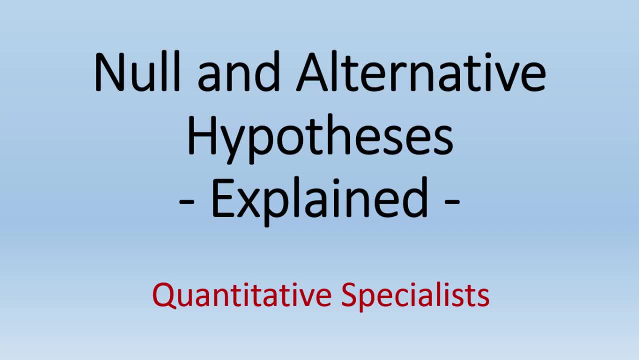 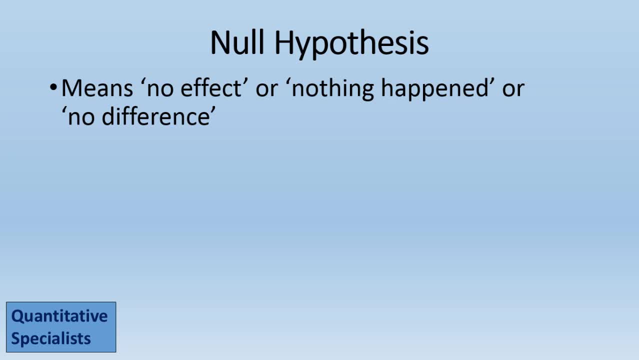 In this video we'll take a look at null and alternative hypotheses. Now, the null hypothesis means there's no effect or nothing happened, or there's no difference. The null hypothesis is often represented by H sub-zero and it makes a statement about the population, not the sample. So in other words, we put 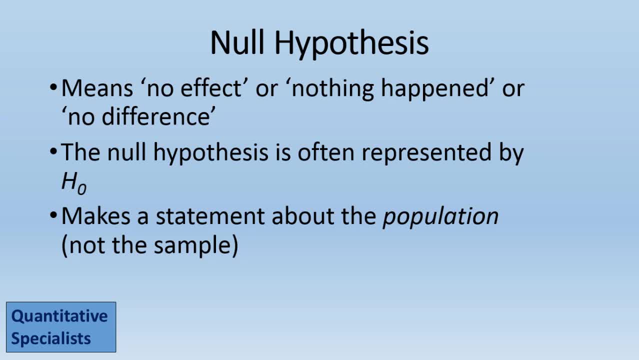 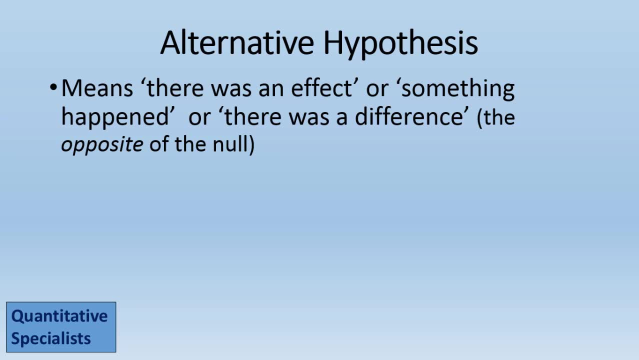 population values or symbols in our null hypothesis. Now the alternative hypothesis is really the opposite. It states: or it means that there was an effect or something happened, or there was a difference. The alternative hypothesis is often represented by H sub-one or H sub-a. 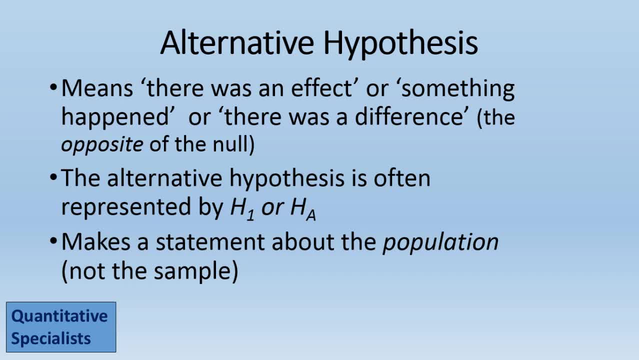 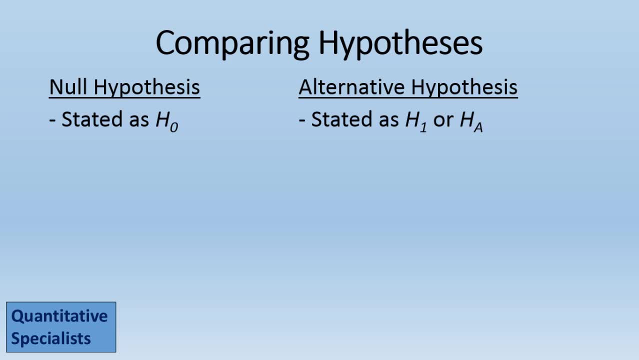 And it also makes a statement about the population, not the sample. So if we take a look at these two side-by-side once again in review, the null is stated by H sub-zero. the alternative is H sub-one or H sub-a. 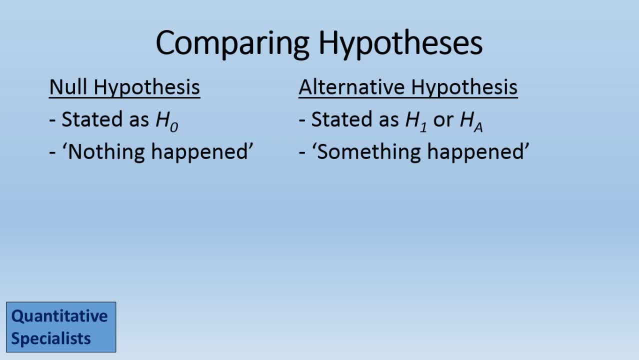 the null basically states nothing happened. and look at the opposite here the alternative states something happened, or the null can state no effect. the alternative states there was an effect and finally the null can state no difference effectively and the alternative would state the opposite: there was a. 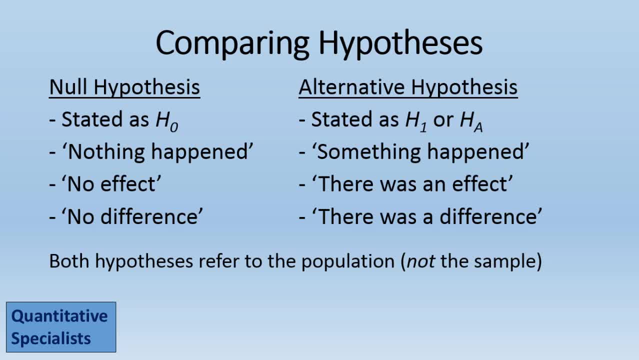 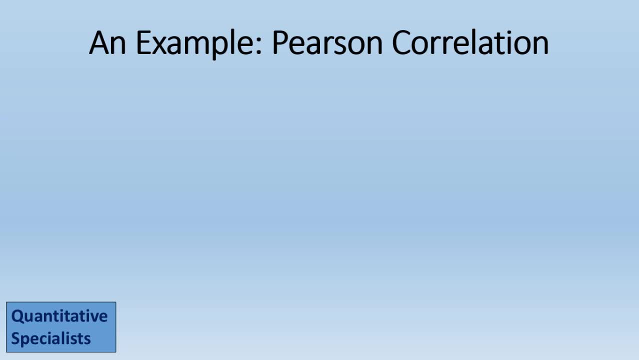 difference And, once again, both hypotheses refer to the population. Let's go ahead and take a look at an example using the Pearson correlation, or Pearson's r. Now, correlation measures the degree of the linear relationship, if there's any at all, between two variables, and it's known as Pearson's r. 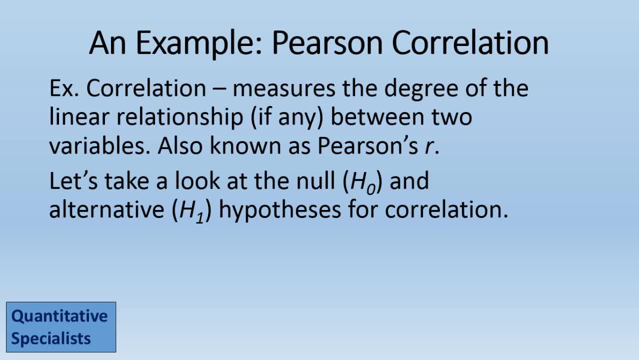 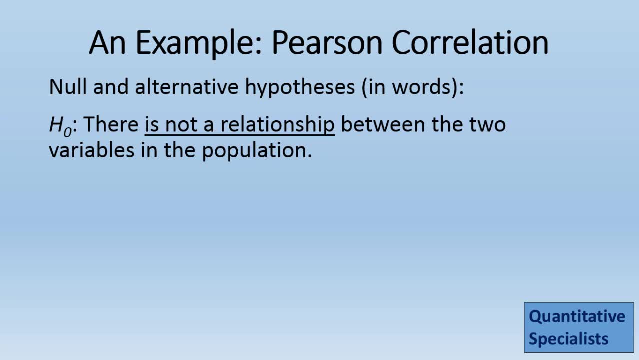 Let's go and take a look at the null and alternative hypotheses for correlation or for Pearson's r here. In words, the null would state there is not a relationship between the two variables in the population. The alternative would state the opposite. it would state there is a. 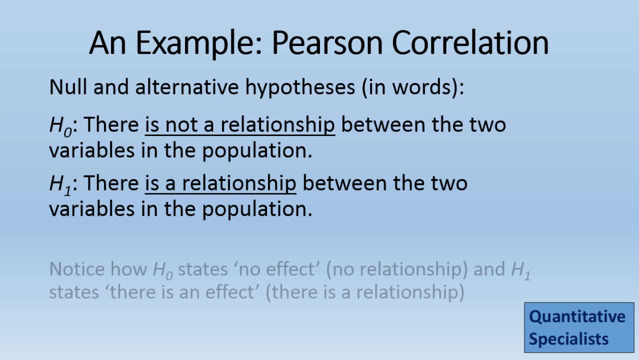 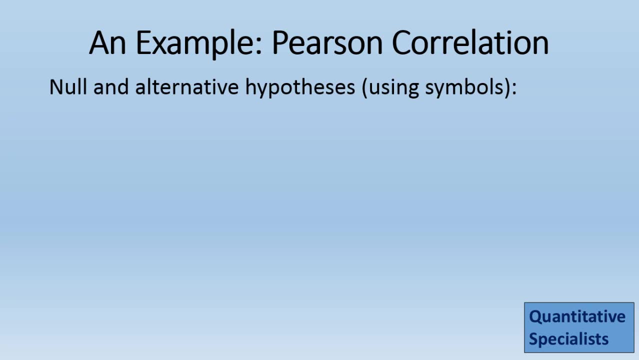 relationship between the two variables in the population. Notice how the null states no effect or there's no relationship, whereas the alternative states there is an effect or there is a relationship. Using symbols, we could say the following: the null and that little thing that looks like a P. 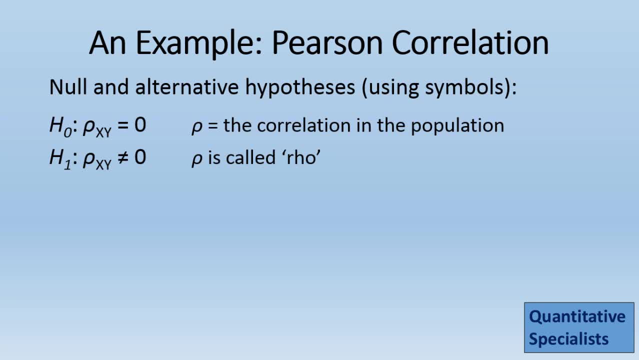 there that stands for rho and it's the correlation in the population. So in this case we would say Null, rho xy equals zero. and then the alternative would say rho xy does not equal zero, Or in other words, the null would state there's no correlation between. 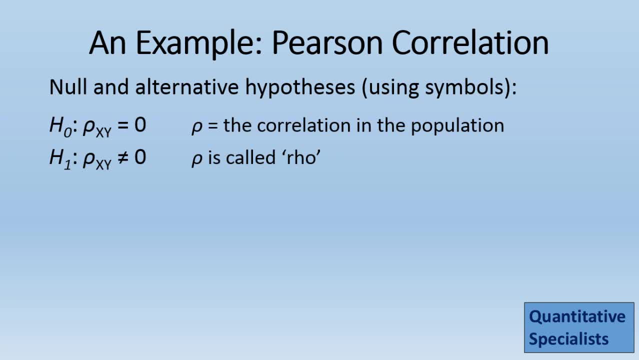 x and y, two variables in the population, whereas the alternative would state there is a correlation between the two variables x and y in the population, and zero here means no relationship in correlation. So when the null says it's equal to zero, it means zero. 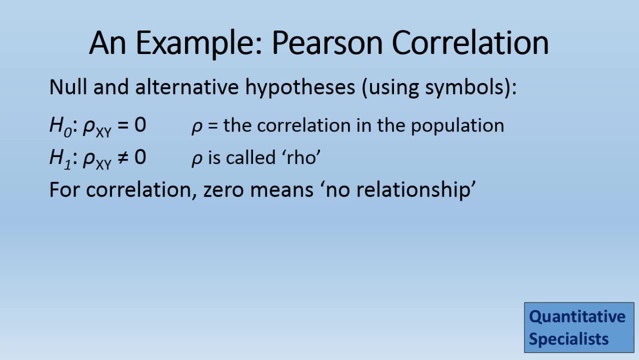 So now you picture it when I show it again. for example, like if a could be positive, So when the null says it's equal to zero, it would have an effect. Will it be positive? equal to zero? it's saying there's no relationship. When the alternative says: 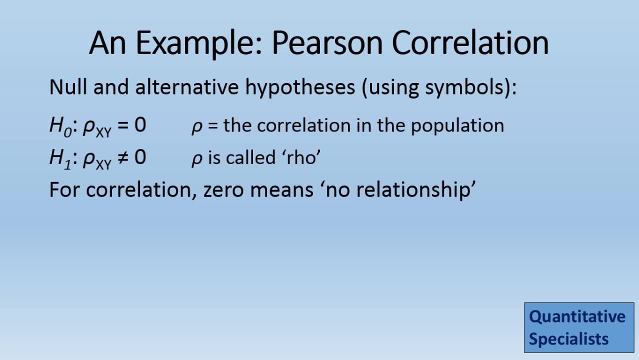 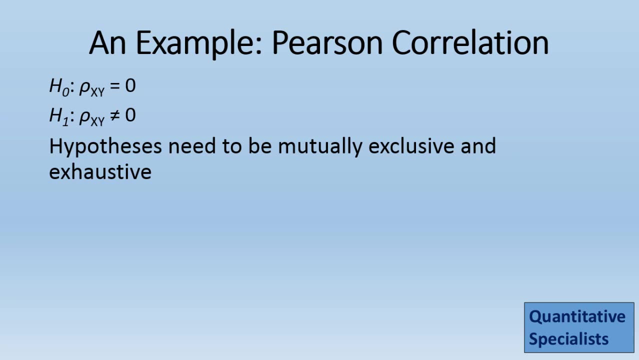 it's not equal to zero. it's stating there is a relationship. So, in review, the null states there's no effect or zero relationship, whereas the alternative states there is an effect or a non-zero relationship. Now hypotheses need to be mutually exclusive and exhaustive. Exclusive means there's no overlap. 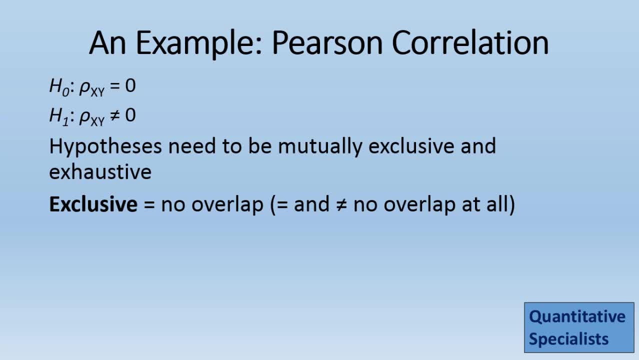 between the null and the alternative. And if you look at our two statements up above, where it says that row xy equals zero, row xy does not equal zero, notice that those do not overlap at all. Equals and not equals are completely non-overlapping. It's either zero, which is the null in that case, or it's not zero. 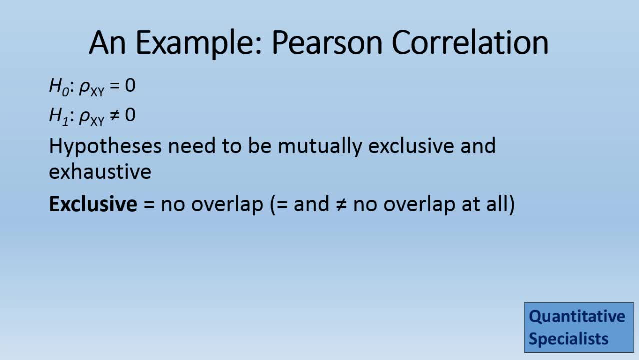 which is the alternative. So they're completely exclusive, they do not overlap. And then exhaustive means they must cover or exhaust all possibilities, the null and alternative when taken together. And notice that they do, as every possible value for Pearson's r is either zero or not zero. So it does exhaust all possibilities. So, once again, 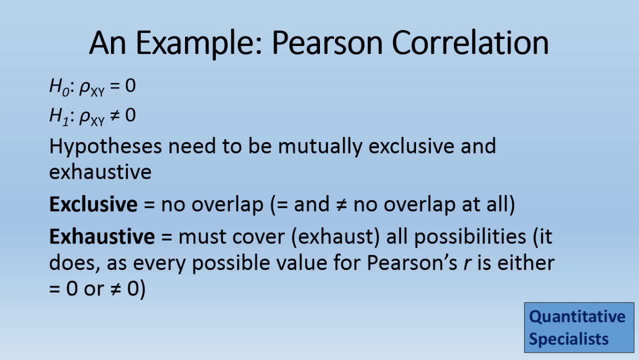 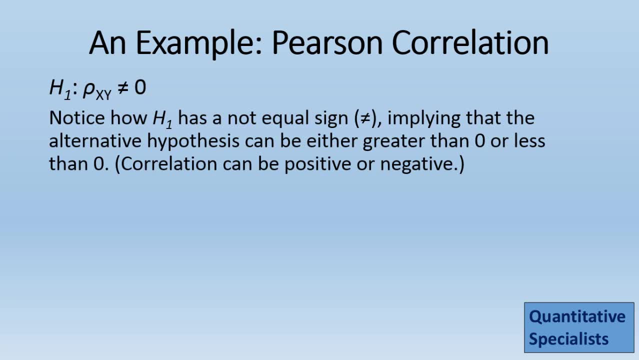 it's exclusive because they don't overlap, and it's exhaustive because they cover all possibilities. Now notice how the alternative has a not equal sign, Implying that the alternative hypothesis can be either greater than zero or less than zero, Or, in other words, correlation can be positive or negative. This is